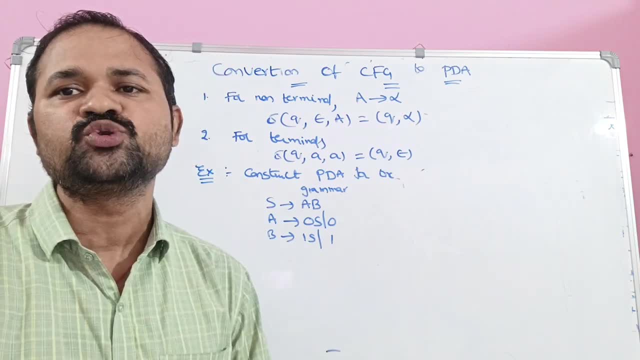 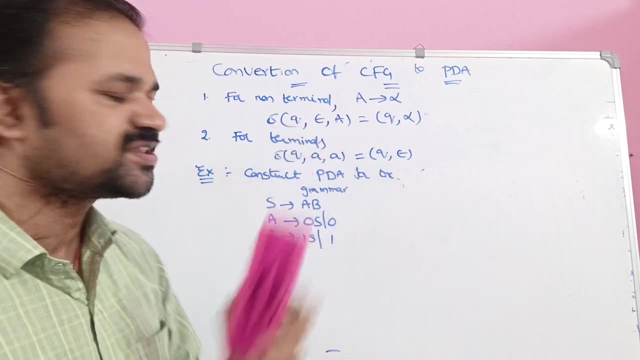 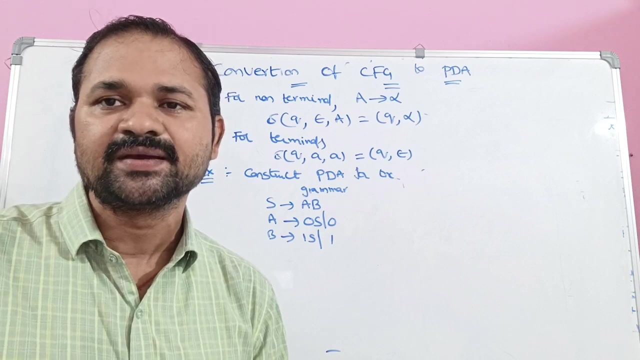 So here, PDA. in order to convert c of g into the pda, we have to follow mainly two rules. the first rule is for the non-terminator, the second rule is for the terminals. so terminals means lowercase letters. so 0, 1 are some symbols: a, b symbols, left parenthesis, right parenthesis plus, minus. 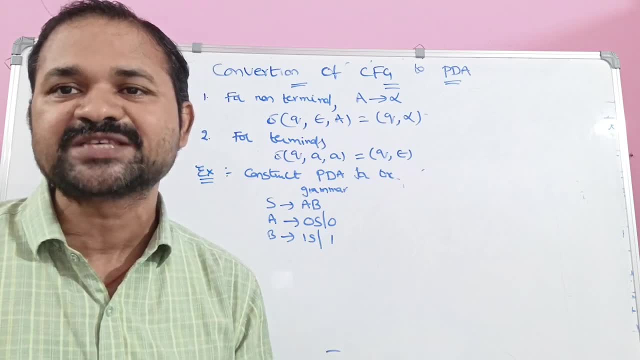 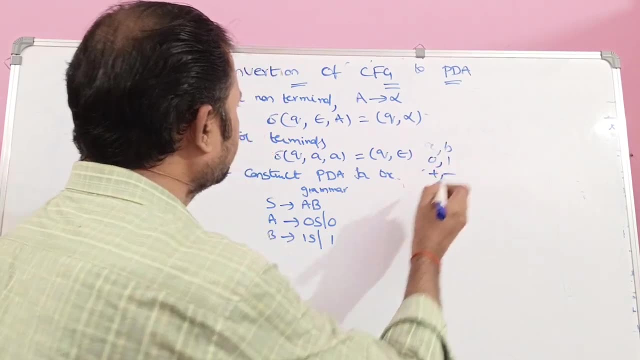 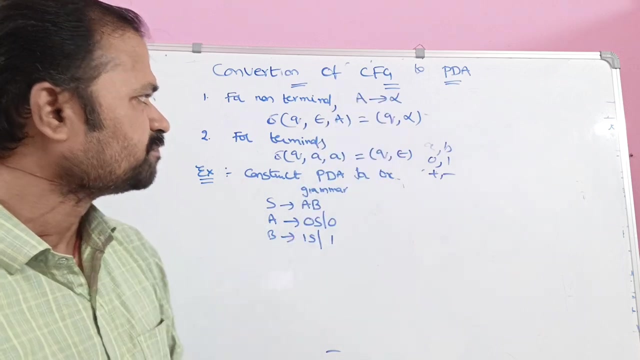 or it may contain lower lowercase letters, small a, small b. so terminals means either lowercase letters or digits or some symbols. okay, various non-terminals means uppercase letters, so that we have a production in the form. a implies alpha, so a means left hand side, but various alpha means: 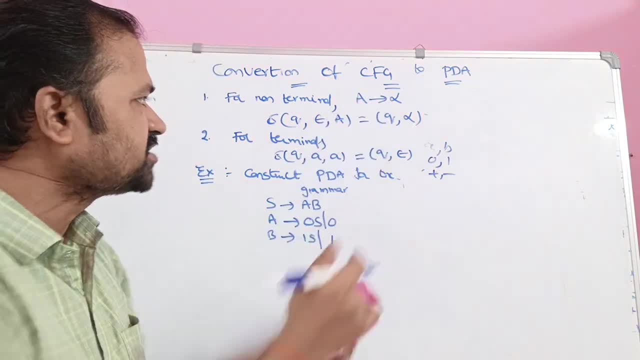 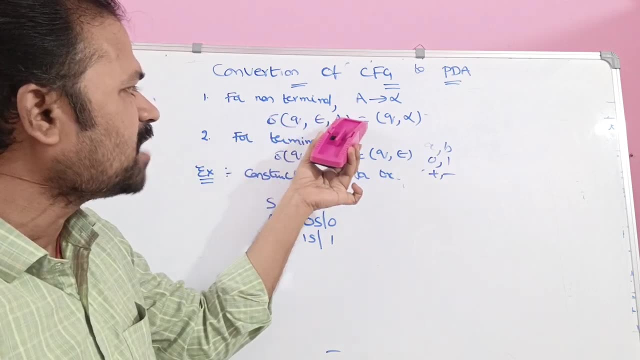 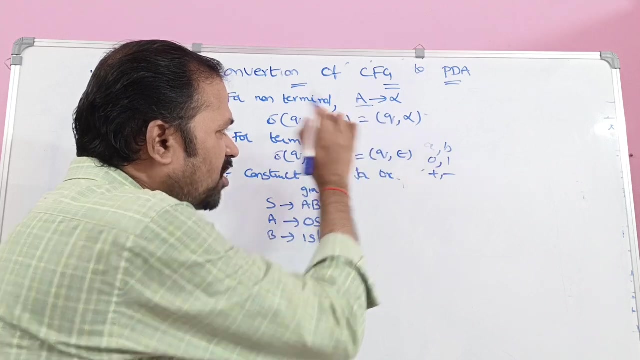 right hand side of the production, then if your production is in this form, then we can write as delta of q: q is the state epsilon comma a is equal to. here we have to apply epsilon. so this a is nothing, but that you, you production left hand side non-terminator is equal to q comma alpha. what is this alpha? this alpha is: 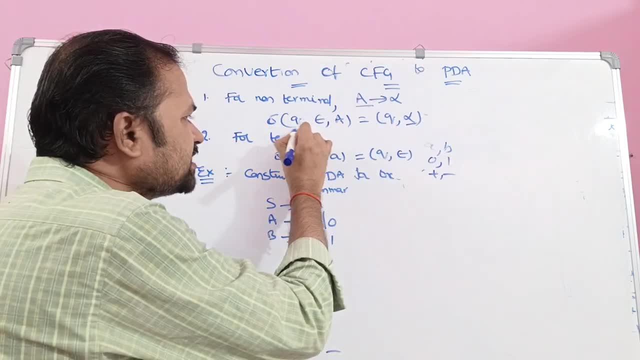 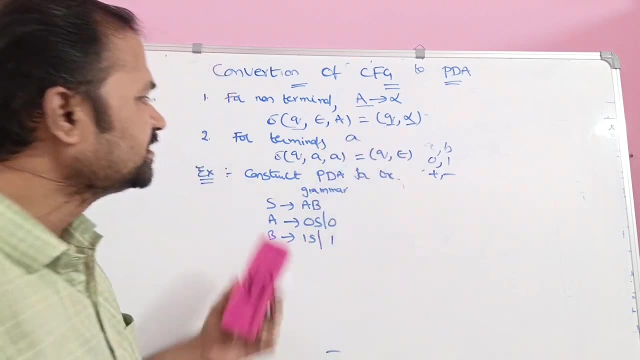 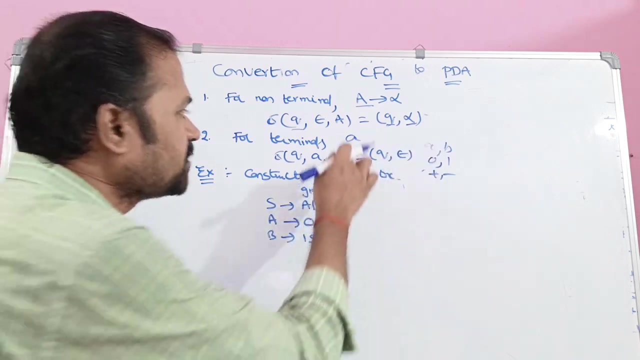 nothing but right right hand side of the production. this q is nothing but that state for the terminal. the rule is like this: if the terminal symbol is a, then we can write as delta of q comma. a comma a is equal to q comma, epsilon, suppose. if the terminal symbol is plus, then we can write as delta of 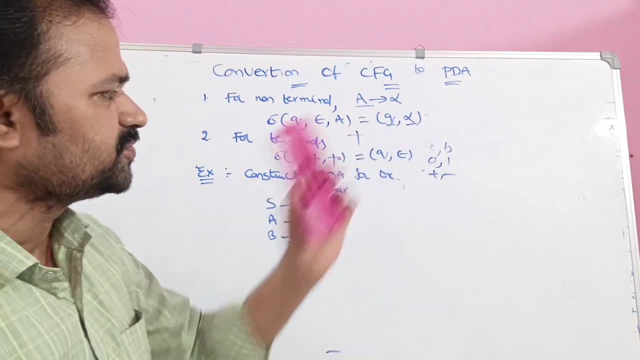 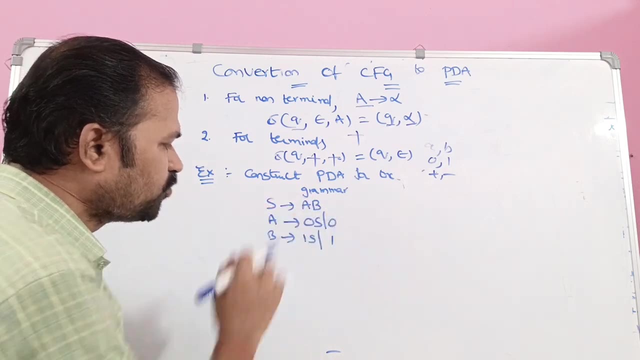 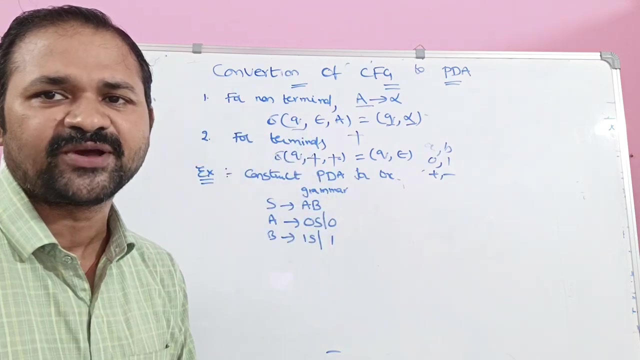 q kama, q gamma plus. kama plus is equal to q kama epsilon. simply, we need to follow those two rules. so here we have 1 for a, we have two productions. three for b, we have two productions, five. so today we have five productions, are there? so, for all the five interactions, we have to write. 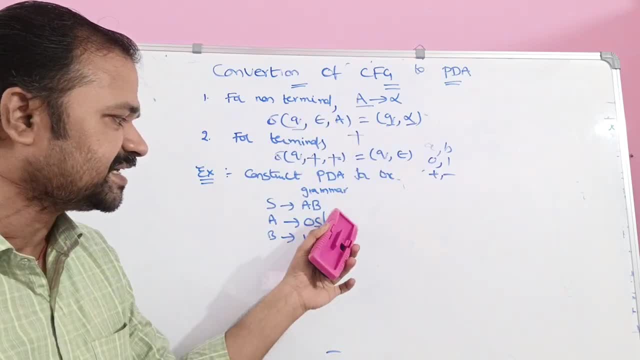 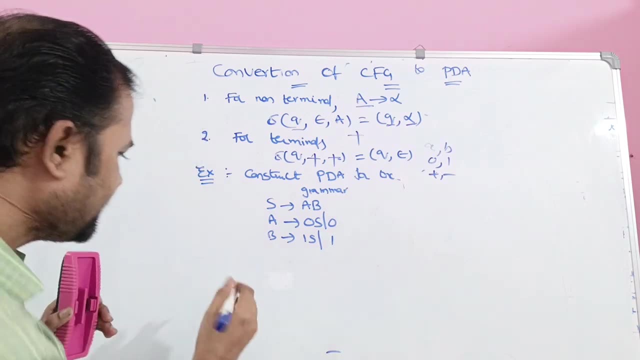 just falling transition functions as well. as we have two terminal symbols, are there zero and one? so for those two also we have to write the production. so first year is: consider the 1st. 2 productions is equal to What is the first production. s implies a, b. Then we can write. as for this production, we can. 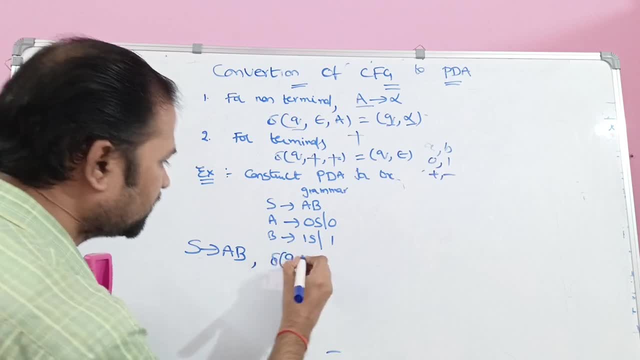 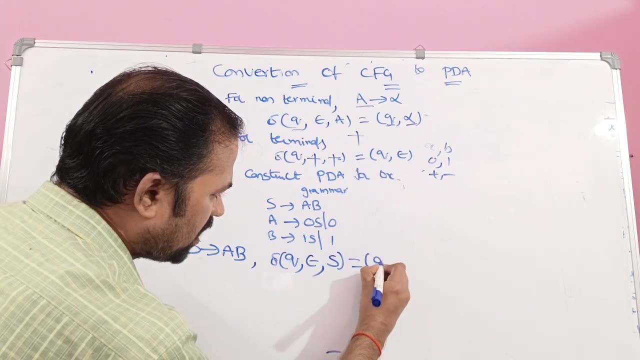 write as delta of q gamma: epsilon gamma. So this: a is nothing but left hand side of the production, s is equal to q gamma. What is the right hand side of the production? a, b. So q gamma, a b. 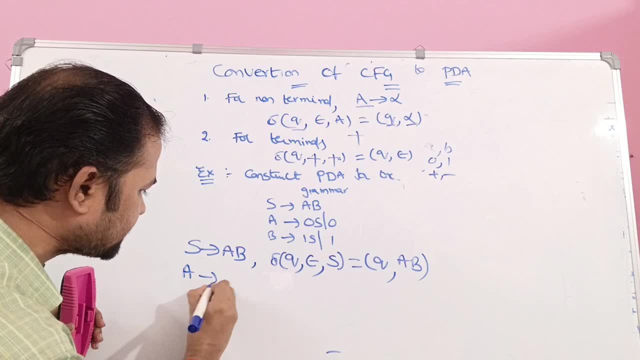 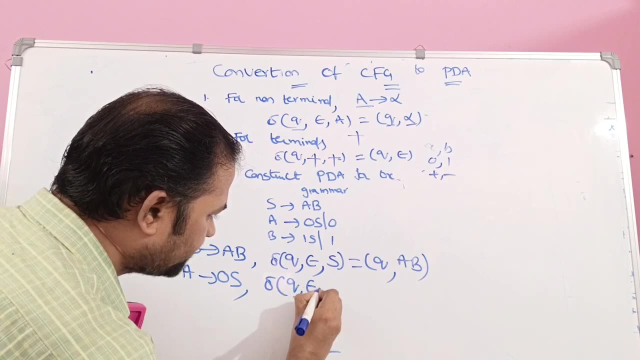 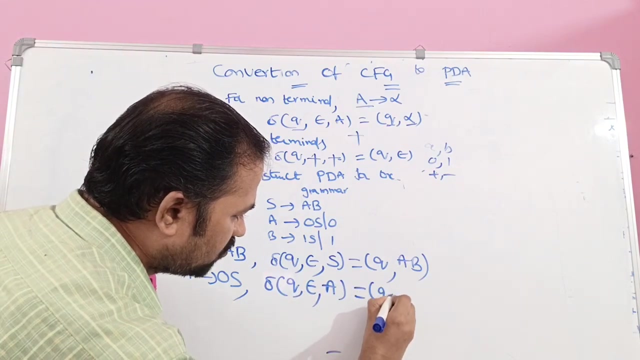 So this is the first function. So next one: a implies 0, s. So for this production we can write as delta of q gamma, epsilon gamma. What is the left hand side of the production, a? a is equal to q gamma. What is the right hand side of the production? 0, s. q gamma, 0, s. 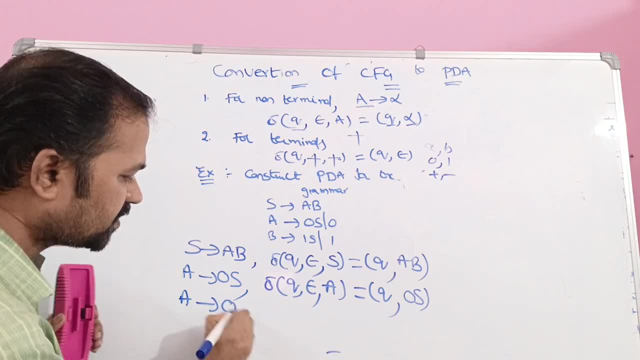 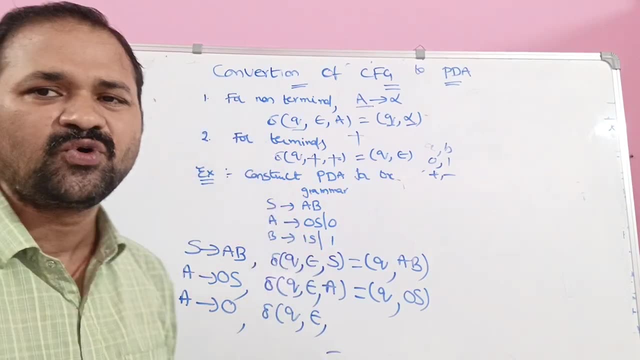 Next, for the next one, a implies 0.. So we can write as delta of delta of q, gamma, epsilon, gamma. Only one state is enough. It may be q or q naught, or q 1, it is your choice. 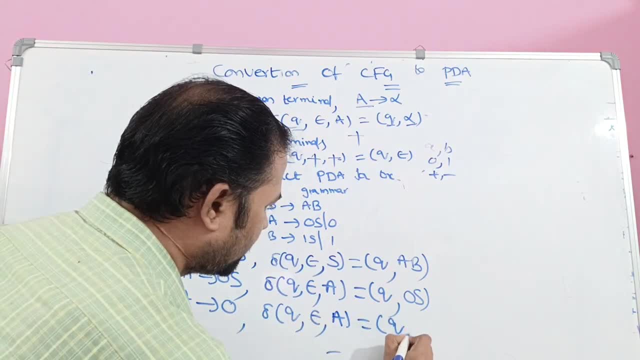 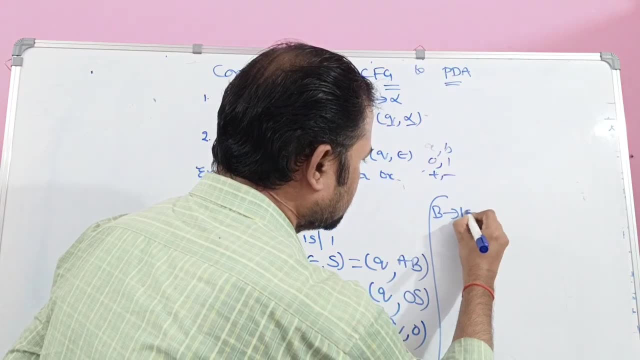 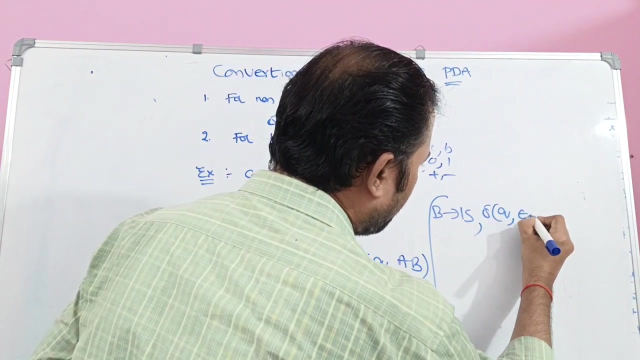 epsilon a is equal to q gamma 0.. Next production: b implies 1, s, So for space constraints I am writing here: b implies 1, s, So we can write here: as delta of q gamma, epsilon gamma b is equal to. 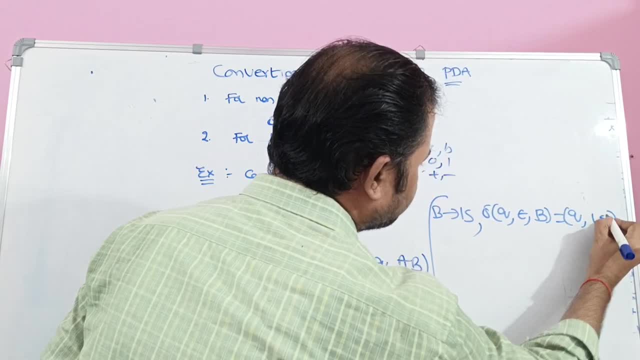 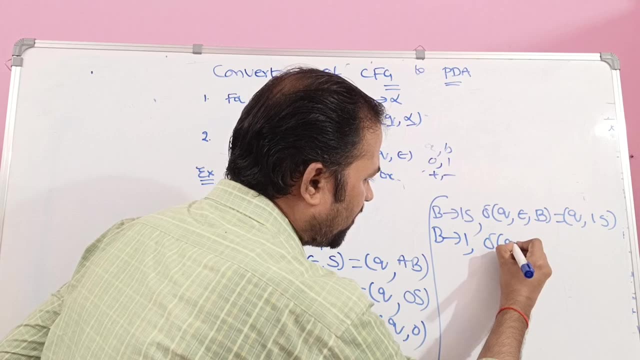 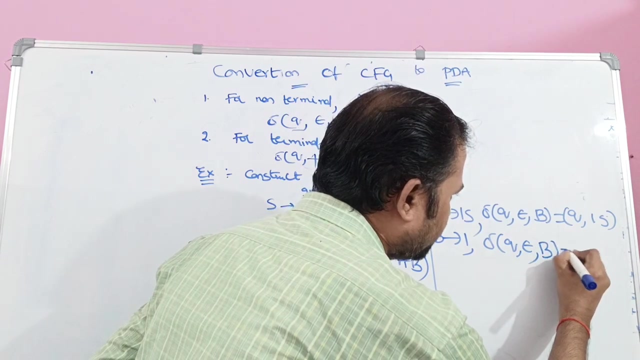 q gamma 1, s. So 1, s means right hand side of the production, So last production. b implies 1.. So this can be written as delta of q gamma, epsilon gamma. What is the LHS here, Not here? b is equal to, so q gamma 1.. 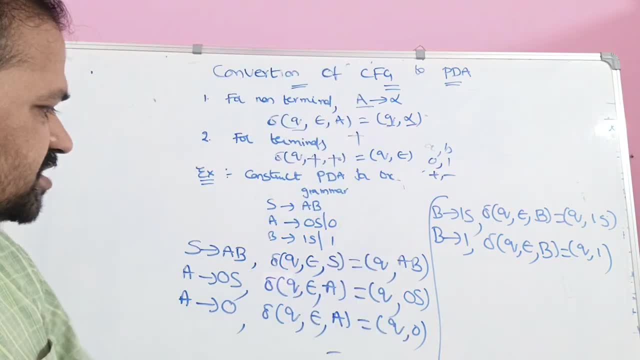 So 1 is nothing but right hand side production. So for all the productions we have written the corresponding transition functions: So a, b, 0,, s, 0.. So q epsilon, q, epsilon s, a, l, a. 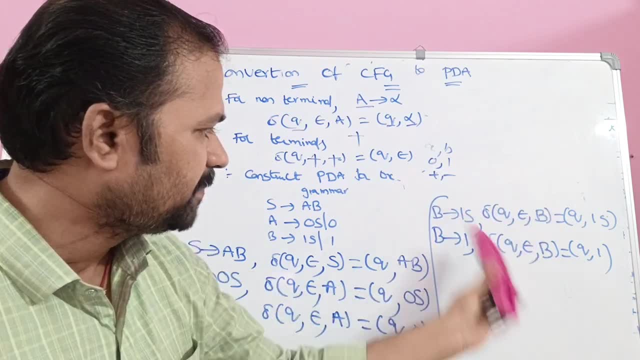 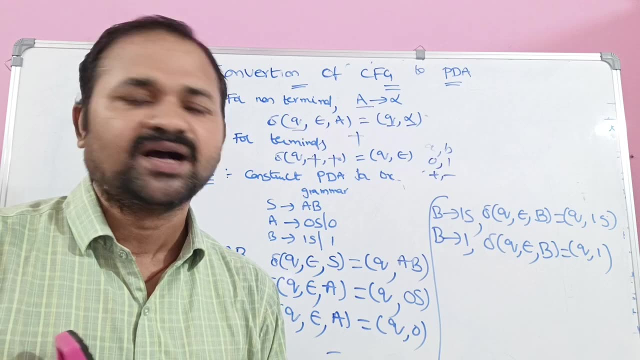 Next: q, q, epsilon b, b, 1,, s, 1.. Next, what are the terminal symbols here? 0,, 1.. So for 0, first let us write the transition function for 0.. So delta of q, gamma 0 is the. 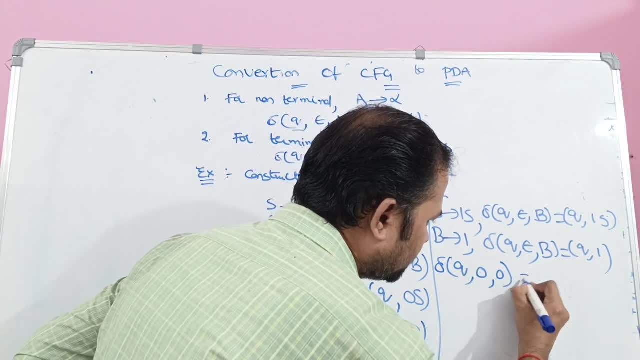 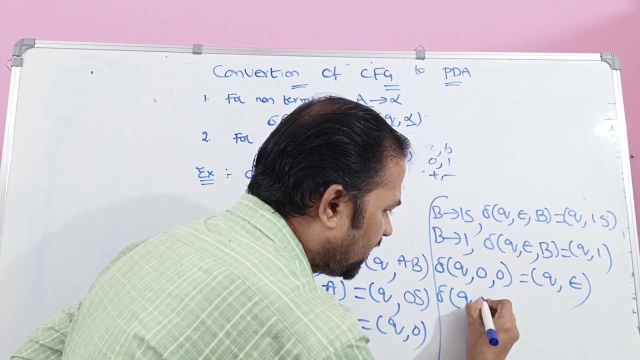 terminal symbol 0 is the terminal symbol is equal to q gamma. we have to write as epsilon. So this is the formula Next delta of q gamma 1. gamma 1 is the next symbol is equal to q gamma. 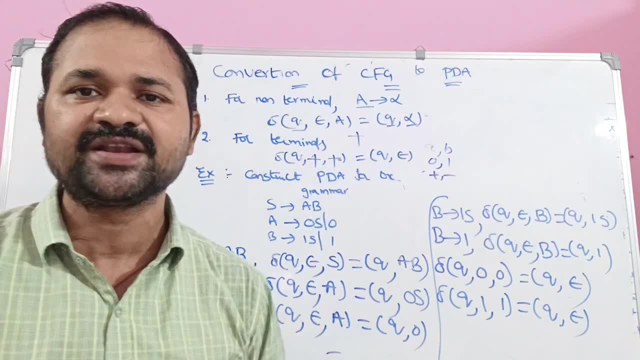 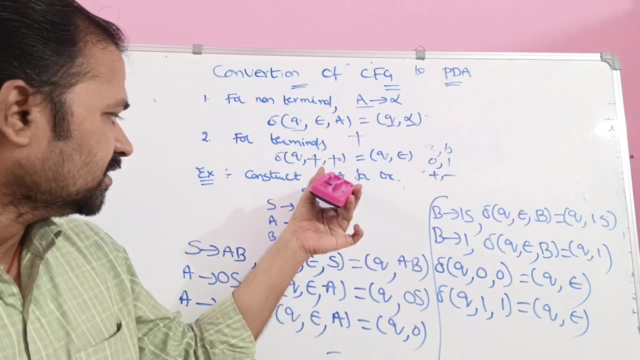 epsilon. So here context-free grammar is given. So for the corresponding context-free grammar we have to find out the PDA. Context-free grammar means mainly grammar productions will be given. So in PDA mainly we have to find out the delta transition functions.